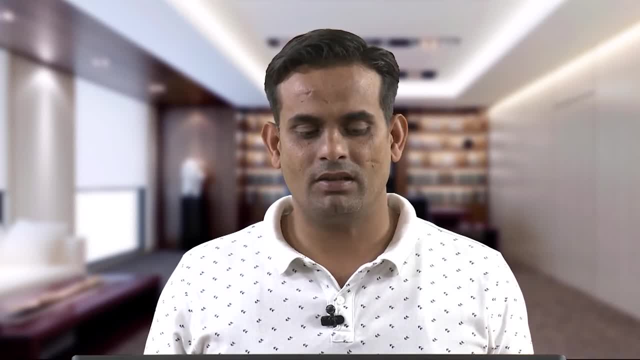 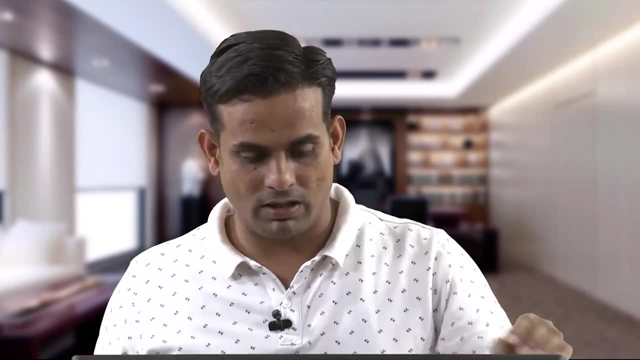 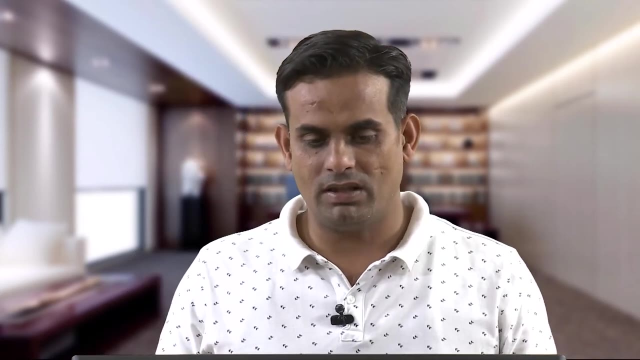 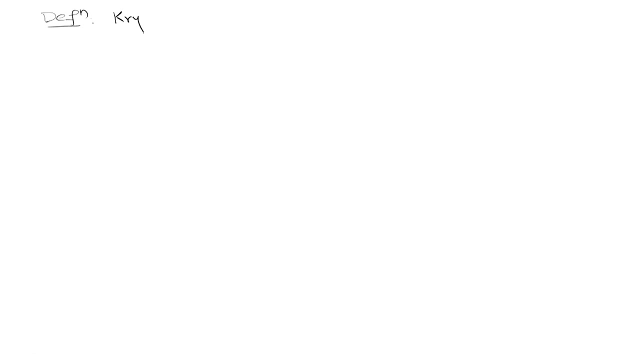 type of non stationary method which is called Krylov subspace iterative methods. So before going to the methods, I will introduce you what we mean by Krylov subspace. So let me write the definition of Krylov subspace. So let a be a. 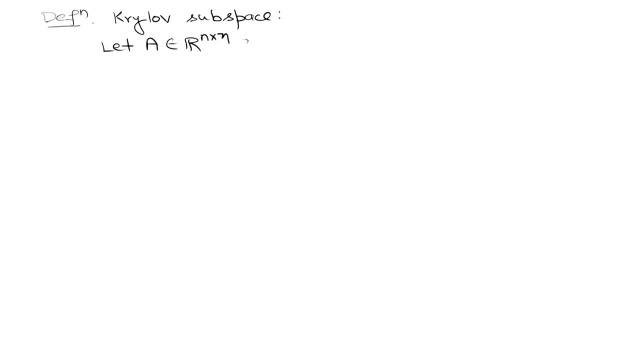 a, n by n matrix having real entries and B be a column vector having dimension n, Then the Krylov subspace, which is denoted as k, j, A, B, is defined as k, j, A, B is defined as it means that z Krylov subspace of A and B is the linear span of the vectors B, A into. 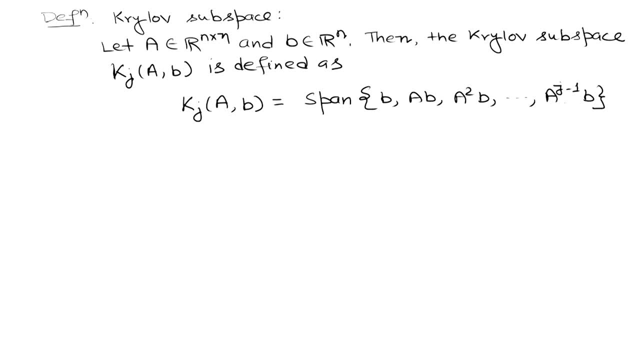 B, A square into B, this way up to a, raise to power j minus 1 into b, And you can observe that again, this Krylov subspace is a subspace of R n because all these vectors are having n components, So all these vectors are coming from the vector space R n. Let us take an example of: 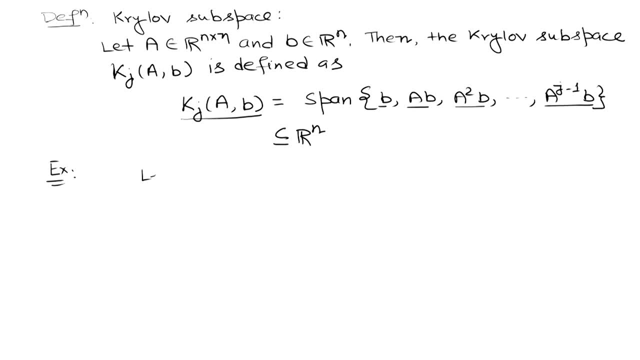 it Let: a equals to 2 1, 1, 2 and b equals to 1 n minus 1. then if I calculate a- b, it will be 2 1, 1, 2.. Multiplied with column vector 1 minus 1 and it comes out to be 1: n minus 1, which is equals. 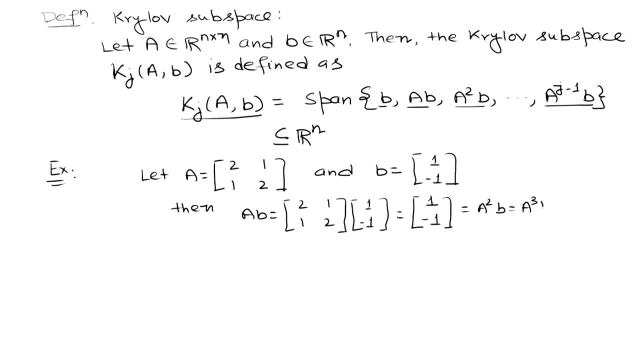 to a square, b equals to a cube p and so on. So here Krylov subspaces, that is, if I write a b as iba will be the linear span. or let me write out this linear span by l of 1 minus 1. transpose Similarly: k 2 a b will be linear span of vector b and a b. So this will be. 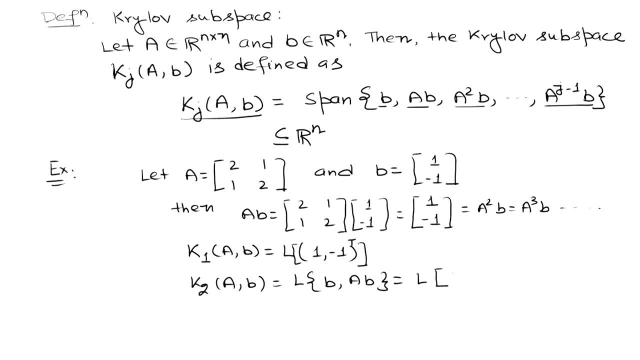 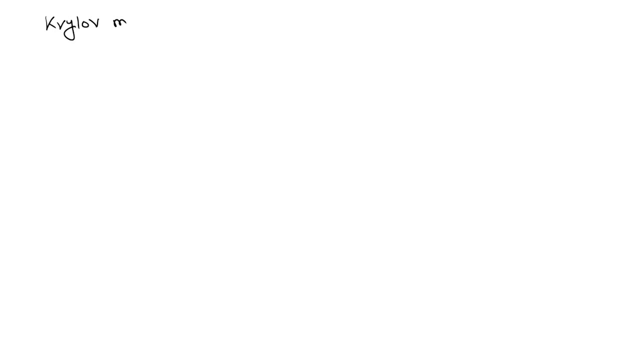 this will be linear span of b and a. b are the same vector, the same vector here. So 1 n minus 1 transpose. So in this way we can define the Krylov subspace. Next I will define Krylov matrix Again, let A be n by n, matrix having real entries and 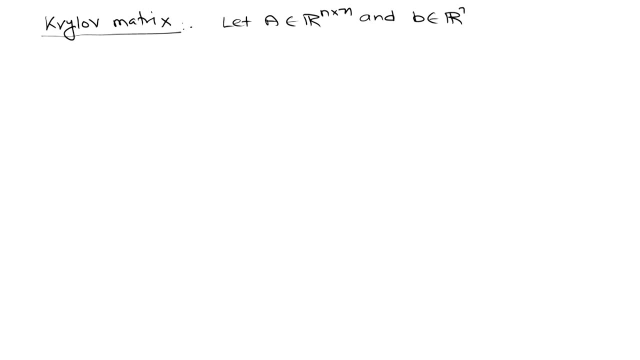 B is a column vector having n component, Then Krylov matrix of z order of A and B is the matrix. So the first column is B, the second column will become A, B and in this way the zth column will become A, raise to power j minus 1 into B. So in this way, if I am having, if I want, 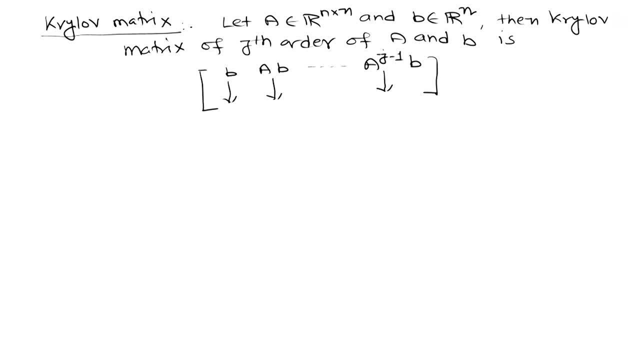 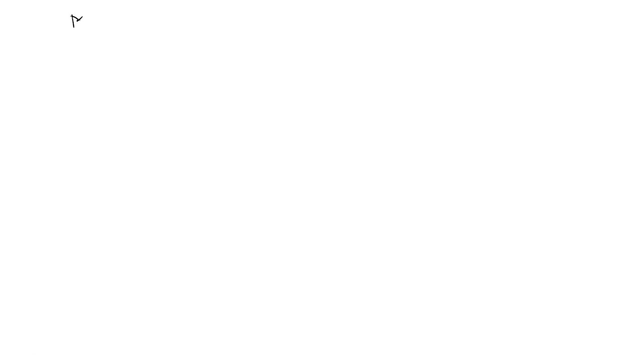 So let us consider. So I want to talk about motivation. So consider the matrix A, which is a 3 by 3 matrix, having entries 0,, 2, 3.. So the matrix will be inside A at the OUT. 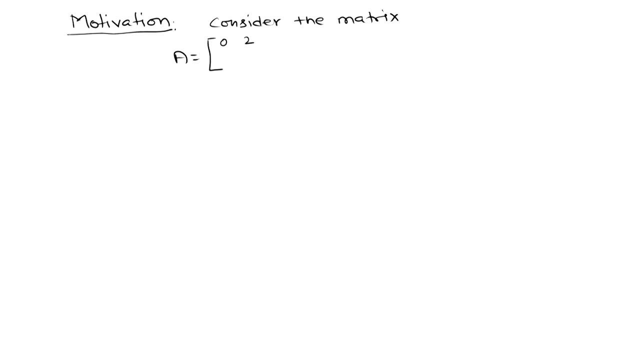 guy and the matrix will be inside A into Z. So this is the matrix q. So in this way we can define the Krylov matrix, and this way we can define the Krylov matrix of a matrix 1, minus 1, 3, 1 and then minus 2,, 2, 3.. Now the characteristic polynomial. 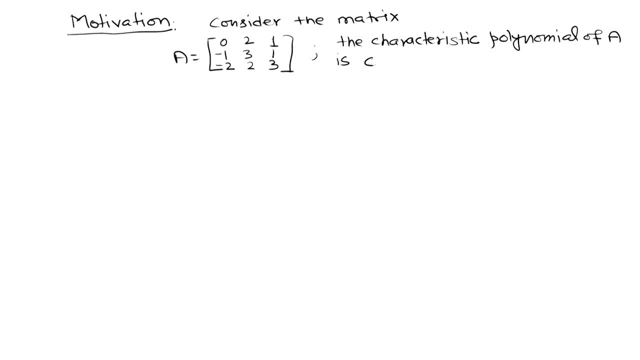 of A is C A lambda, which is just determinant of A minus lambda I, and if I calculate it, it comes out to be a polynomial in lambda of degree 3, which is: lambda cube minus 6, lambda square plus 11 lambda minus 6.. 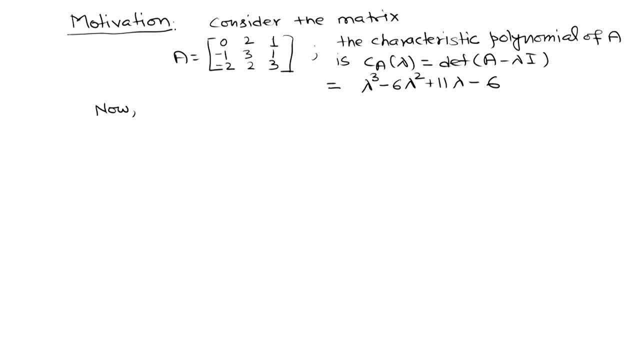 Now by the Cayley-Hamilton theorem we have. so what? Cayley-Hamilton theorem tells us that every matrix satisfies its characteristic equation. So it means I can write A cube minus 6, A square plus 11, A minus 6, I, where I, is an identity matrix. 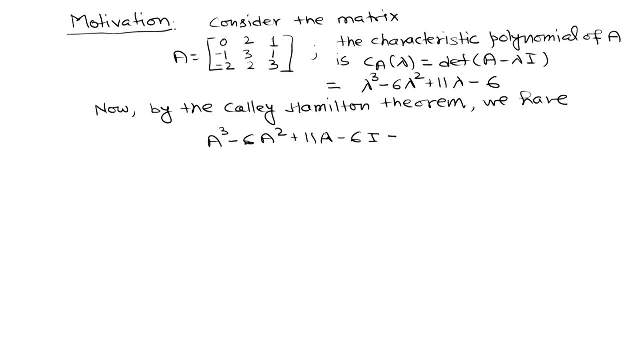 of order: 3 by 3 in this case equals to 0, which is general matrix of size 3 by 3, or I can write from here: if A is an invertible matrix, Then A inverse equals to 1 by 6, A square minus 6, A plus 11. I. So what I have done. 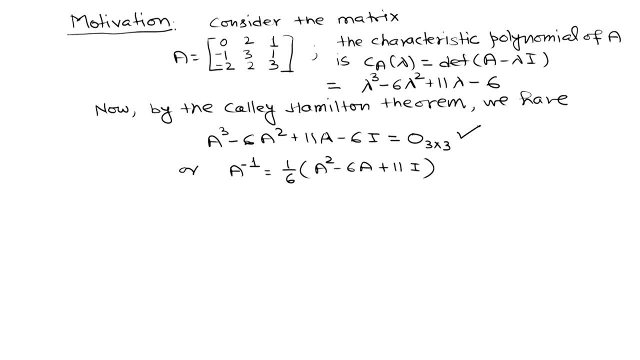 I have multiplied this characteristic equation, means in terms of matrix, by A inverse, and I have written in this way: Let us say, this is a polynomial of matrix And this is also the polynomial of matrix A. Now, so from here I can say that the inverse 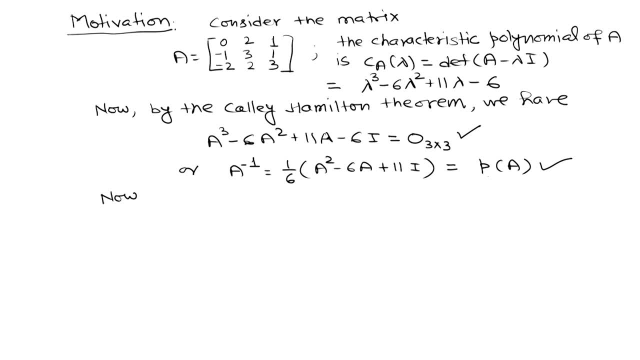 of A can be expressed in terms of: as a polynomial of matrix A. Now if we have a system x equals to B where A is an invertible matrix, then the solution of this system can be written as X equals to A, inverse into B, which I can write in case of this matrix 1 by 6 A square. 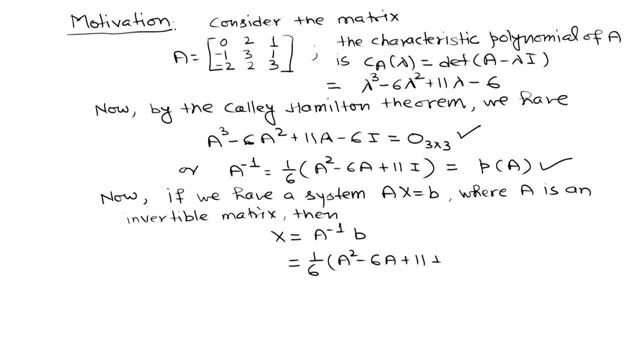 minus 6 A plus 11 I into B, which is nothing, just P of A into B. If I do it, what I will get? I will get minus 6 A square into B. minus 6 A B plus 11 B. If you see this particular. 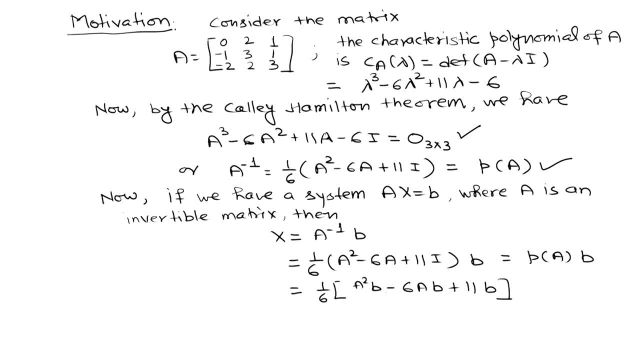 vector that is A square B minus 6 A, B plus 11 B. it is a vector column vector having three components, So 3 by 1 vector. this is just linear span of, So hence the solution of the system. A, X equals to B is a vector from the Krylov subspace. 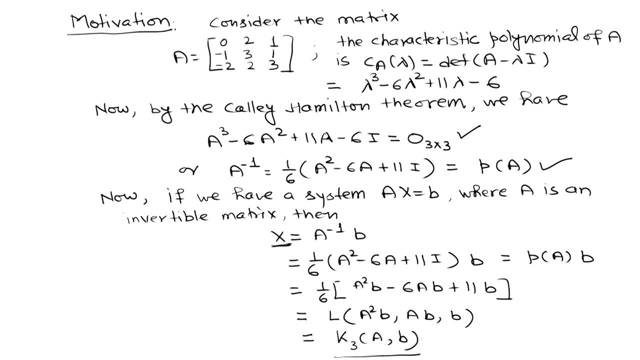 K, 3, A, B. So that is the motivation of using Krylov subspace for solving iterative system. Now what I want to mention here: if A is a large and sparse matrix, but it is non singular, then Krylov subspace method is a very effective method for solving linear system. We will 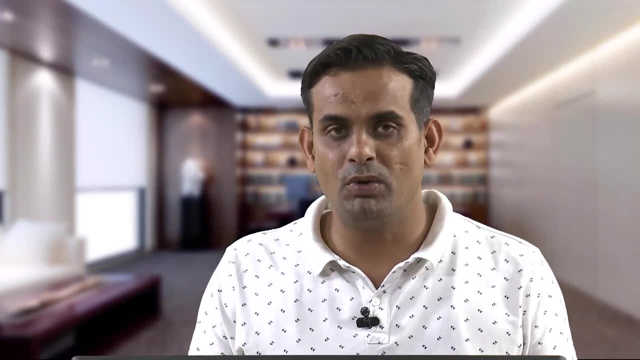 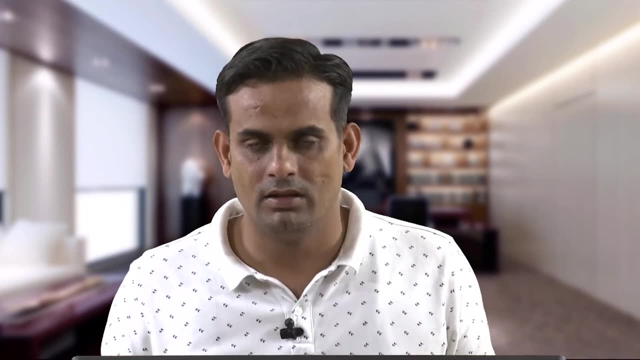 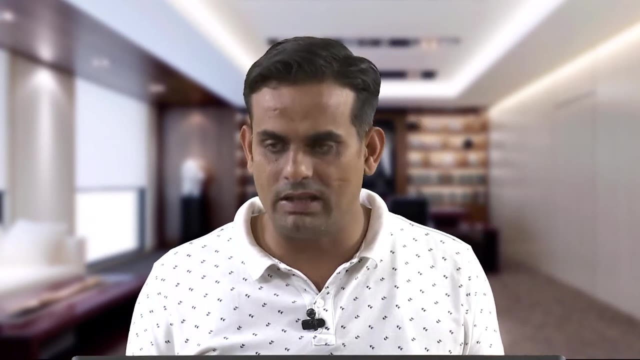 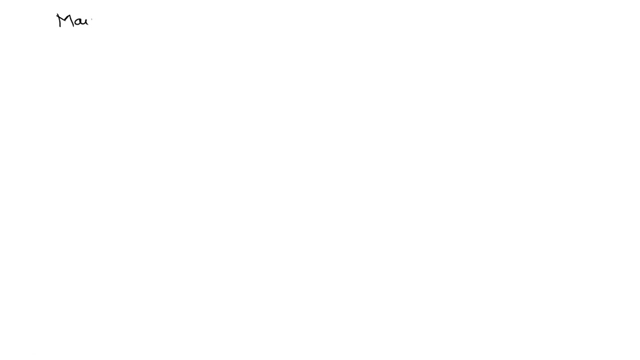 get the solution with less computational complexity as compared to any other iterative method, standard iterative methods like Jacobi and Gauss-Siedel or some direct method. So this is the motivation of using Krylov subspace method. One more thing I want to write about this: that is a main result. So we can summarize: 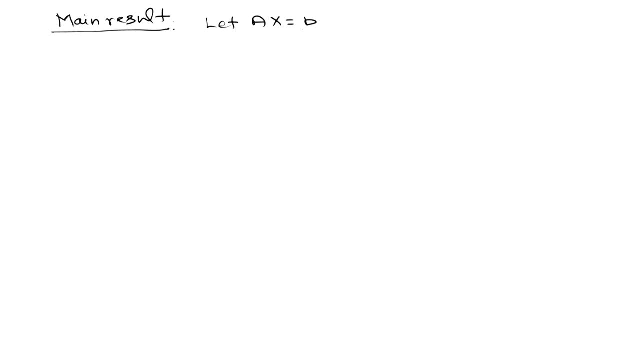 this main result as let. A, x equals to B, B. a linear system where A belongs to R, n by n and B is a vector from n-tuple real vector. So we can summarize this main result as: let. A- x equals to B, B, a linear system where A belongs to R, n by n and B is a vector from n-tuple real vector. 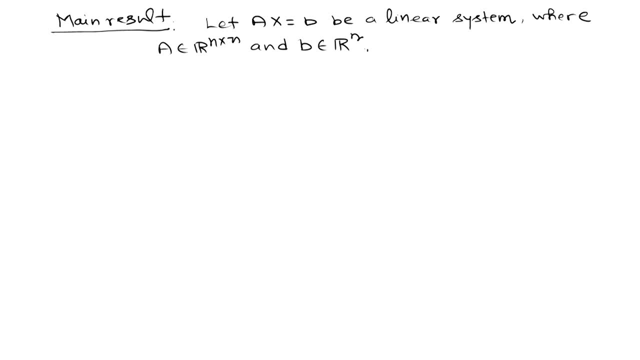 So we can summarize this main result as: let: A, x equals to B, B, a linear system where A belongs to R, n by n and B is a vector from n-tuple, real vector j equals to 0, to m minus 1. alpha j, t, j, where alpha 1, alpha 2, all these alpha 0, alpha 1 up to alpha m minus 1, all these are scalars, all these are real numbers. basically. 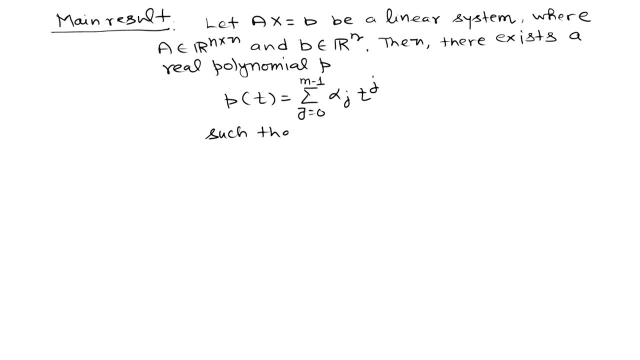 Such that the solution of system x equals to B can be written as x equals to, to P a into b, and this can be written as: j equals to 0, to m minus 1 alpha j a, j b. here this is the P a. Now it is not necessary here that m equals to n means the degree of 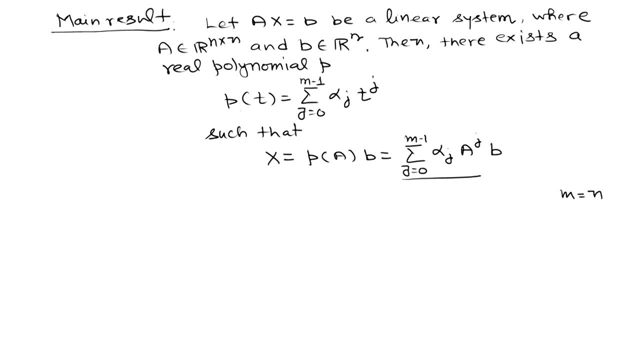 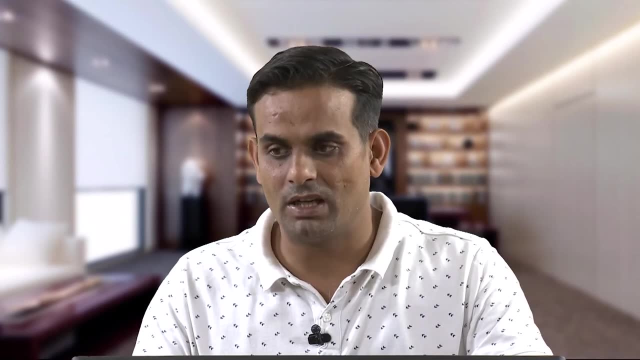 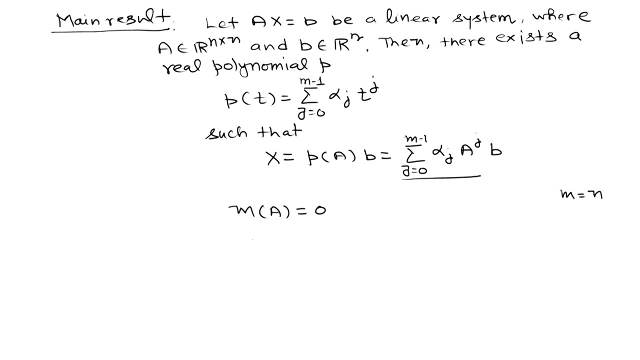 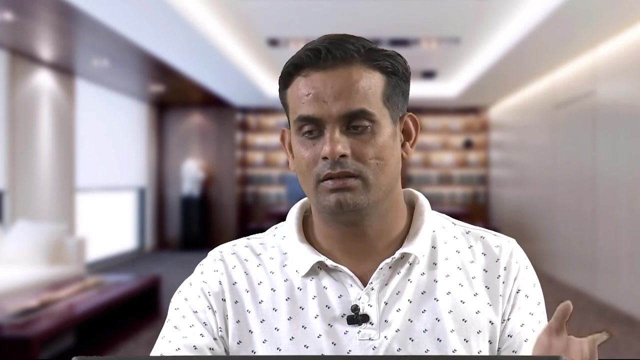 the. this polynomial P, t will be a characteristic polynomial of the matrix A. One of such case is the use of minimal polynomial, because minimal polynomial of a matrix A is also 0 and from there we can use, we can find out A inverse which is having fewer degree, sometimes compared. 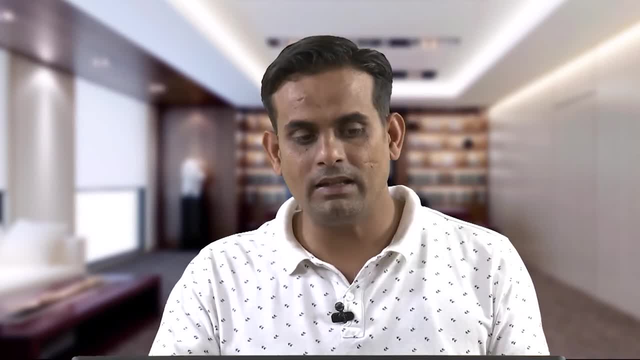 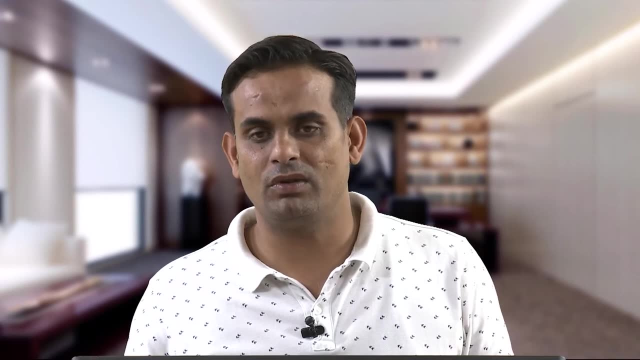 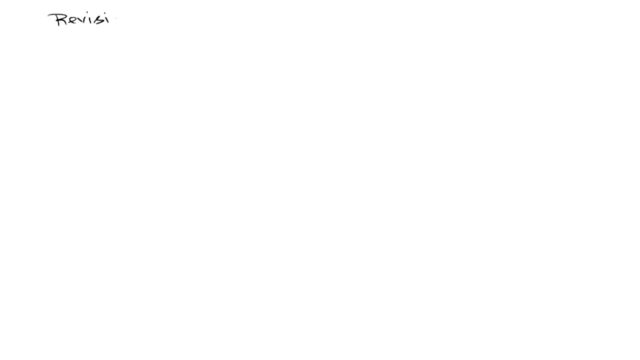 to the characteristic polynomial And that is why I was saying that these methods are quite effective and having less computational complexity. Now just try to formulate method using this subspacing. So let me revisit Kylov subspaces. The Kylov subspace K, j, a, b is the column space of the Krylov matrix. 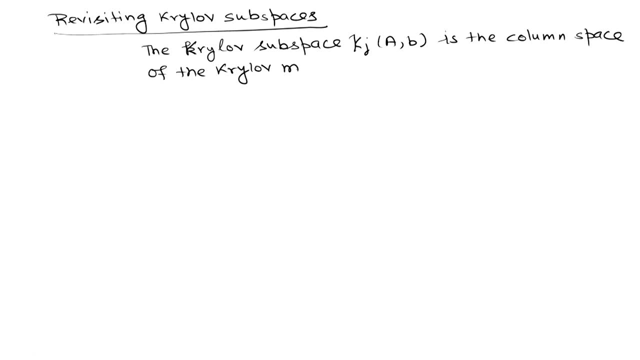 Which is quite obvious because the columns are of Krylov. matrix is nothing, just the vectors b, a into b, a square into b, up to a, raise to power, j minus 1 into b. Now for solving a linear system. we want to choose. 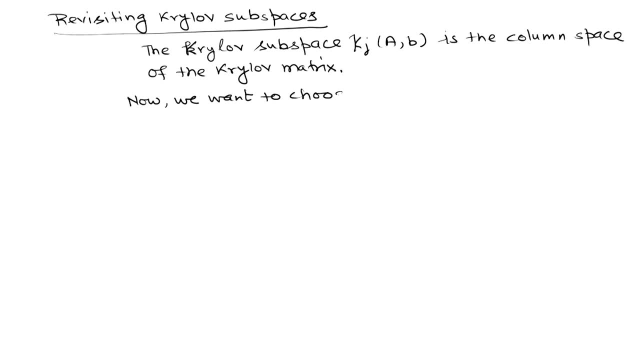 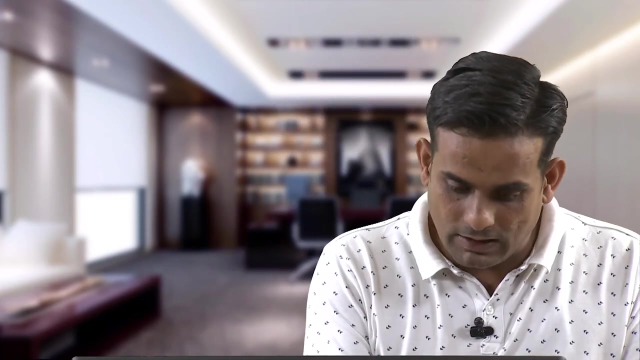 The best combination as our improved x j in jth iteration, If you are having x j minus 1.. Now there are various ways of defining this best, or there are various ways of choosing x j in jth Krylov subspace of A and B. So let us see what are those way. 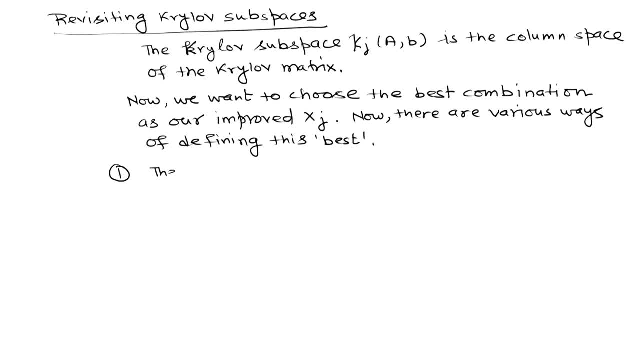 So the first way is the residual R j, which is nothing, just b minus A, x j. So choose x j in such a way from the Krylov subspaces K, j, a, b, such that the residual R j is orthogonal. So R j should be an orthogonal vector to K j, a b means R j is orthogonal to all vectors. 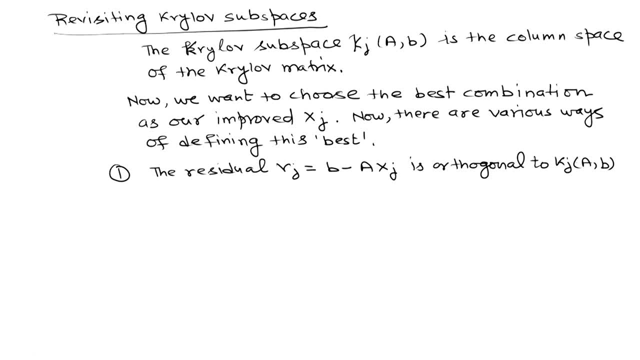 from this Krylov subspace. If you use this strategy, then we will have a method that is called conjugate gradient method, or, in short, CG method. The second strategy is the residual: R j has x, j minus 1.. So the second strategy is the residual: R j has x, j minus 1.. 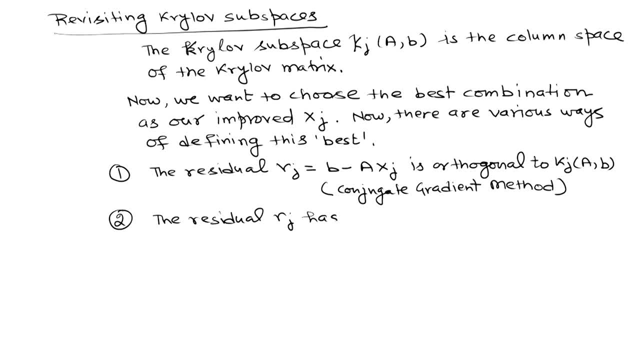 The third strategy is the residual R j has minimum norm for x j in K, j, a, b. So if we follow this strategy, then the method name is: we got another Krylov subspace iterative method that is called G M R E S method. 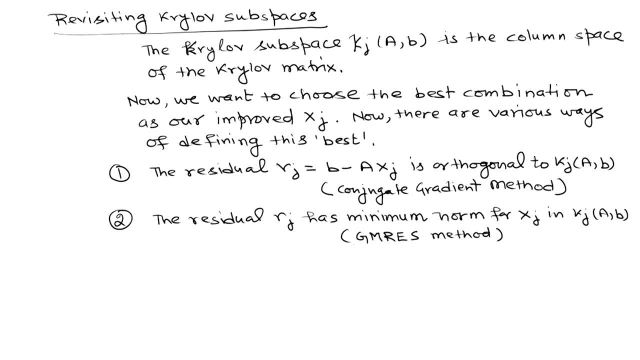 So this is gradient method for minimum with minimum residual. The other way of defining this space may be R, j, which is the residual, is orthogonal To a different space: K, j, a, t, b. So here you just notice that instead of a I am having Krylov subspace of a transpose. 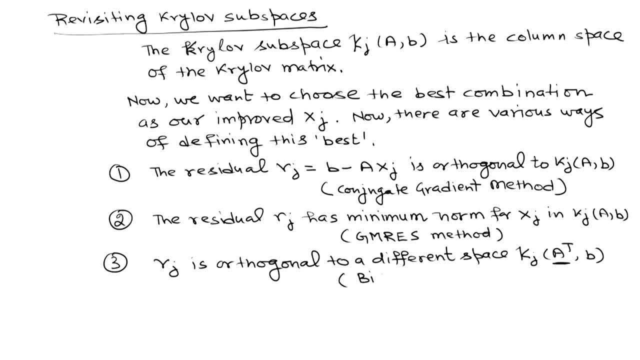 n, b. This method is called biconjugate method. The next strategy is: the error E, j has minimum norm, So the error in jth iteration has minimum norm, And this is the strategy we follow in a method called SIM L Q. 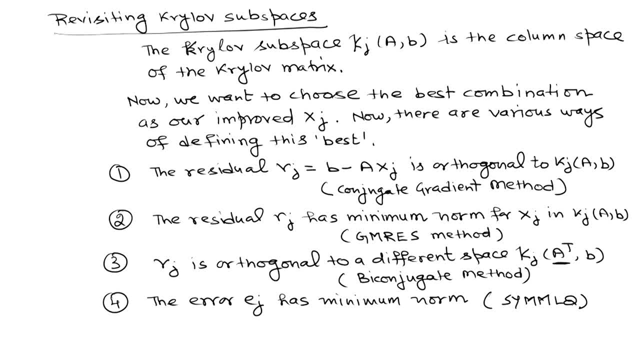 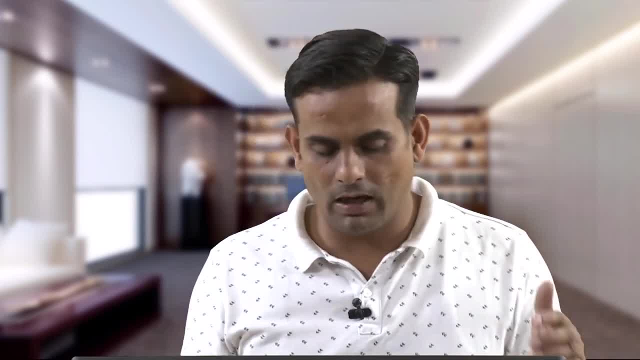 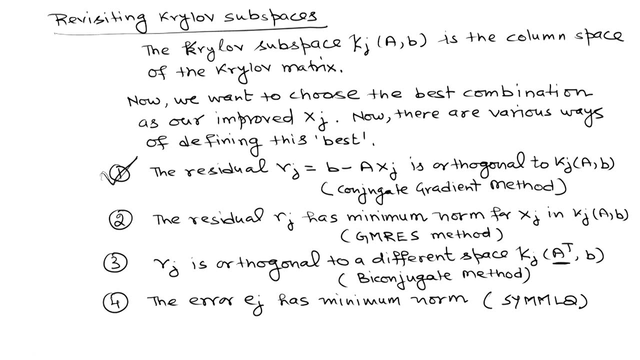 So in this way we are having these four Krylov subspaces method based on defining this best in different way. There are other methods also In this course. I will focus on this method because if you know one method, you can follow. 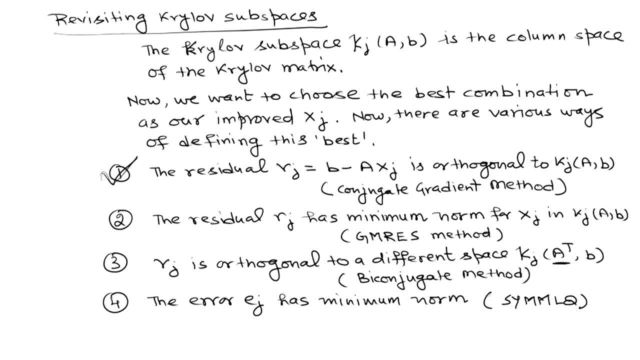 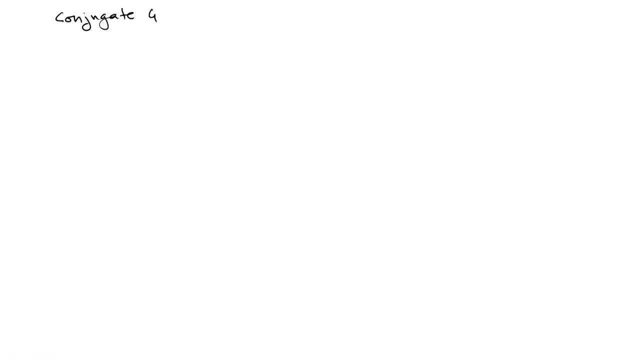 the other methods from the literature In a simple manner. So let us learn what is conjugate gradient method. 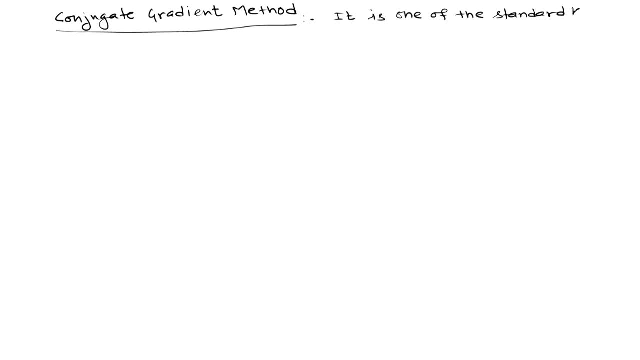 subspaces method, which is used when the system is large and sparse. but the matrix, that is, the coefficient matrix, A is symmetric and positive, definite, Like in the case of steepest descent method. So it is A is SPD in short. So let us go. 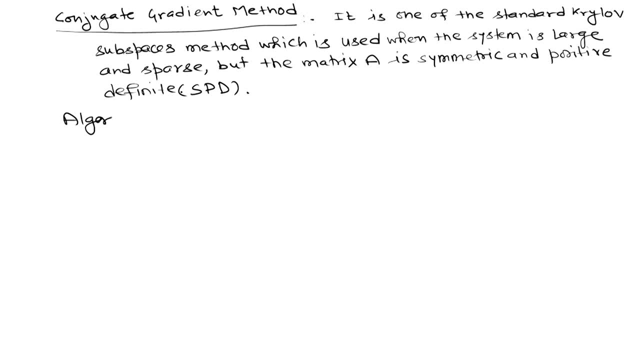 to the algorithm how this method executes. So input is a symmetric and positive definite matrix. say Which is the coefficient matrix of the linear system: x equals to b, right hand side vector b and initial guess at 0 because it is a non stationary iterative method. 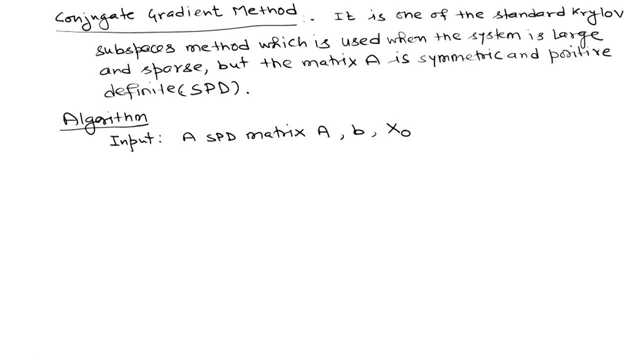 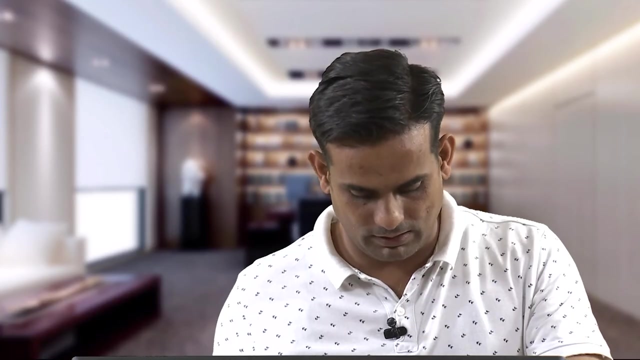 So we need some initial solution. in first step, compute r0, R0, R1.. R0 x r1.. R1. R0 x r2.. which is b minus x 0, and it is same as in case of steepest descent After computing. 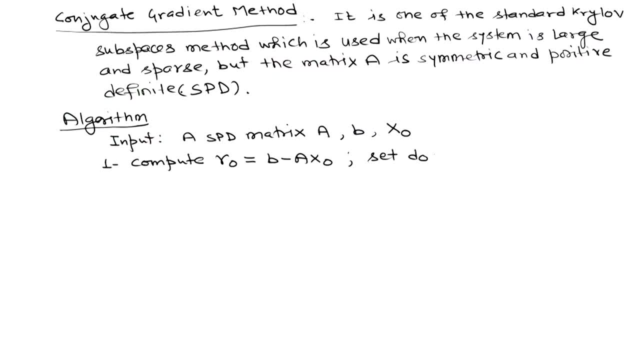 this set the such direction in the initial iteration, as d 0 equals to r 0, which is again similar to steepest descent. Now for k, equals to 0,, 1,, 2 until convergence. do calculate alpha k, that is the step length, which is again same as in case of steepest. 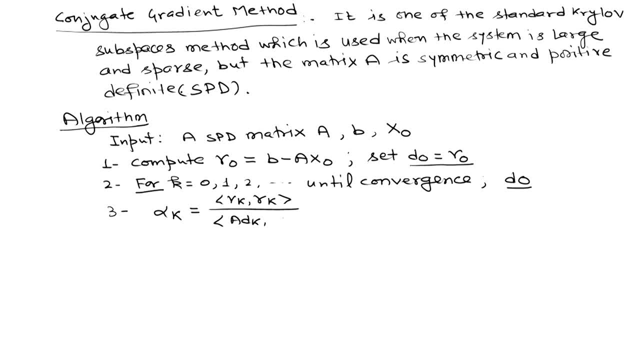 descent in initial iteration, Then it will change because later on we will make the change in that such direction. Then fourth step is compute r k plus 1, x k plus 1 equals to x, k plus alpha k, d, k, the same iterative equation as we are having in steepest descent. Next from here: 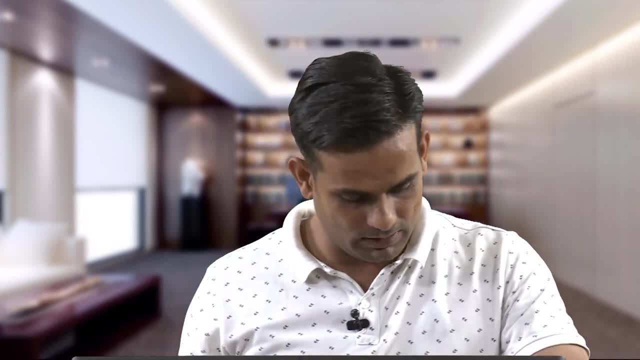 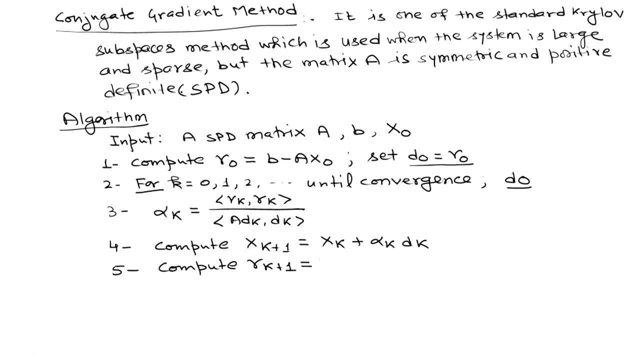 this method will differ from steepest descent method. Compute r k plus 1, which was b minus x plus 1 in steepest descent, but here it will become r k minus alpha k, d k. Then if r k plus 1 equals to 0, then stop. else calculate beta k, which is r k plus 1, r k plus 1 upon. 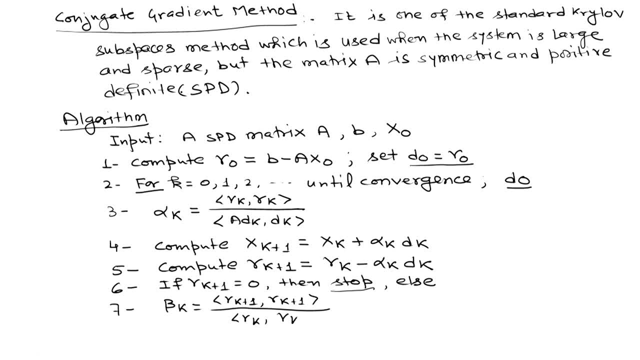 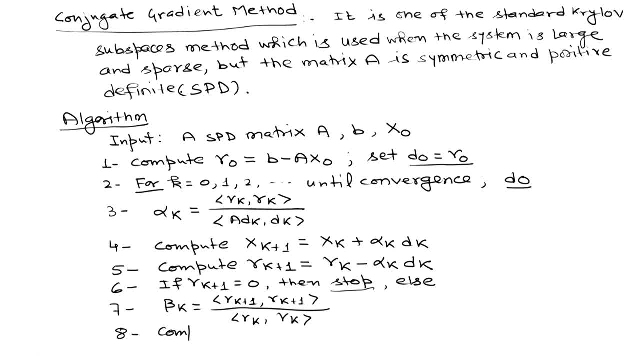 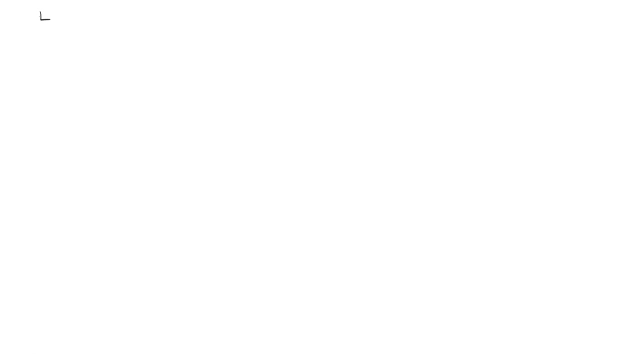 Then what you do: Compute d k plus 1 as means next search direction: r k plus 1 plus beta k, d, k, and then end of your for loop. So this is the complete algorithm for conjugate gradient method. If I need to explain this method vertically, then let us have a quick look on it. So let 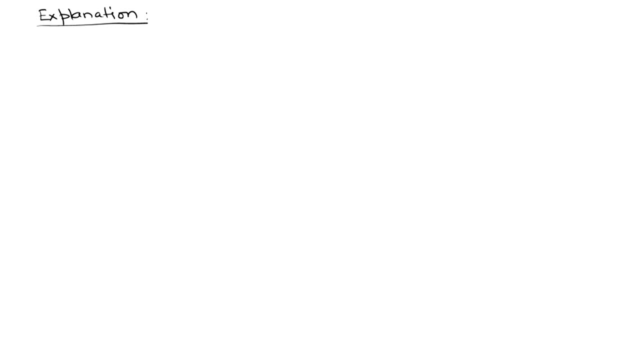 us have a quick look on the explanation of this method in vertical sense. So the conjugate gradient algorithm returns approximations means in different dictations of the gradient. So x, j, that is the solution in jth iteration as a vector of the sum of initial solution. 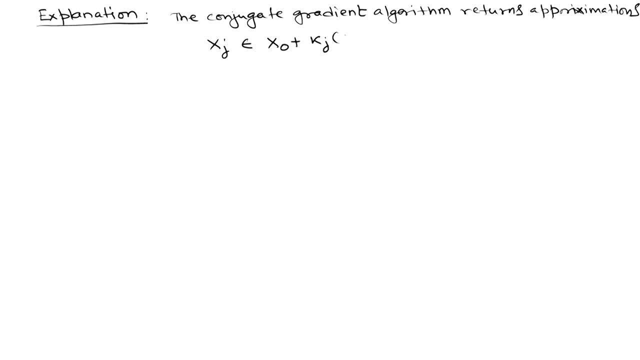 plus a vector from jth Krylov subspace of a and r 0. And this is true for j equals to a 0,, 1,, 2 and so on, such that the error in jth iteration with a norm a should be minimum. 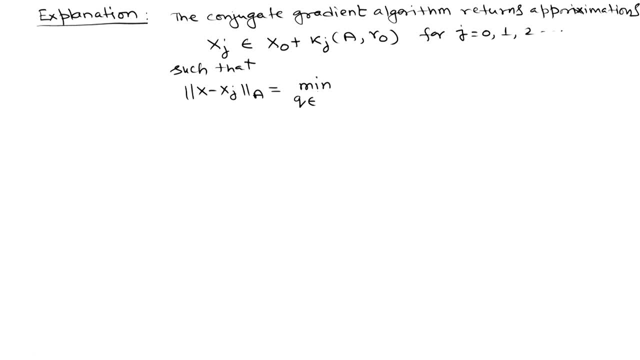 over a vector q which is from a polynomial of degree j minus 1.. And the corresponding error at untuk i minus a, q. a in to x minus x, 0, where the norm is define as button x, t, x, t, x for a given vector x, 0.. 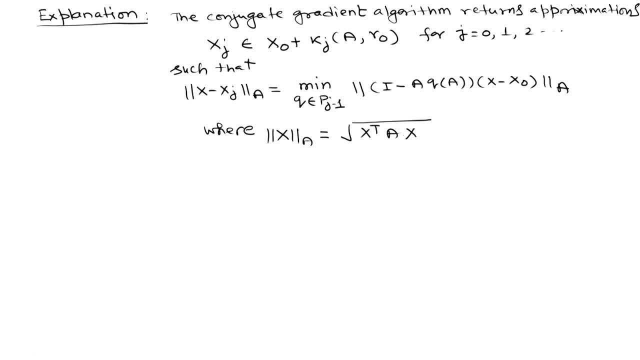 x, t, x, x, t, x. for a given vector, x 0.. x 0,, 2, 8 and so on till x 2. here this is equal to x 0.. So this is local root of the orbital of x. we have x 1 minus and because x is a double power out by X, this is the 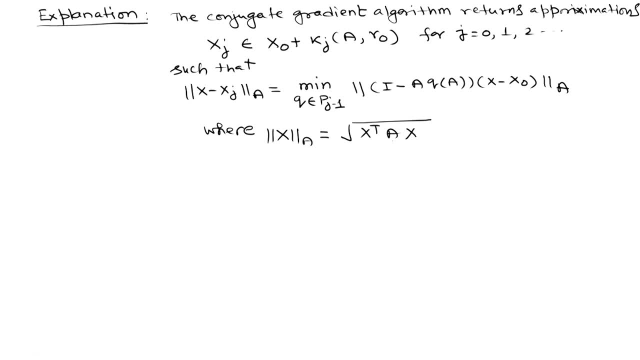 integral of two be�� as x bar about x. we have already drawn So\. So it is the norm induced by the matrix A. Now, if we look, first step of this method means, for going X 0 to X 1, what we are having: X 1 equals to X 0 plus alpha 0, R 0.. Now this: 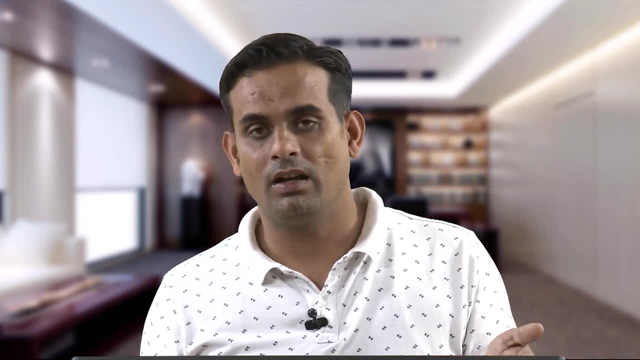 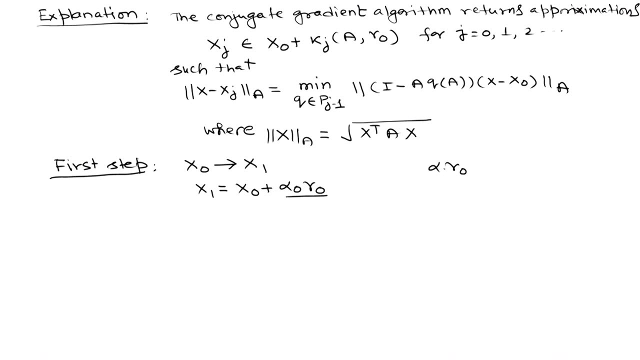 alpha 0. R 0 is a vector in K of 0 A of R 0, R 0 is alpha 0. R 0 is a vector in K of 0 A in this Krylov subspaces, because this Krylov subspaces will be having vectors. R 0 means. 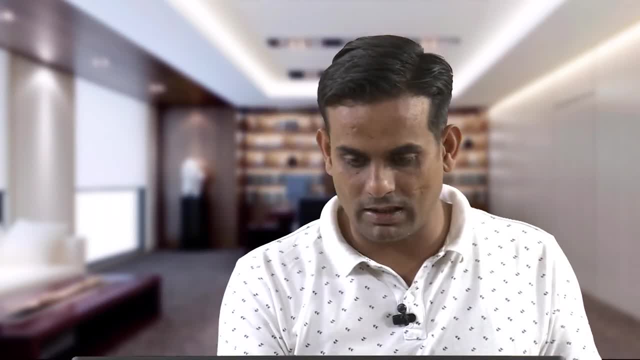 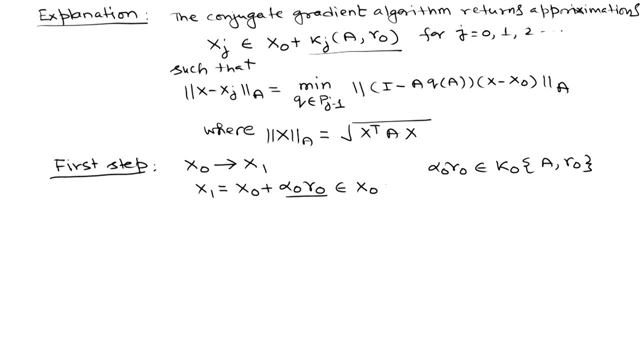 scalar multiple of R 0.. So it is X 0 plus this one. Now this belongs to X 0 plus K 0, K 1, sorry, not 0.. alpha 0 will become r 0, r 0 upon again if I write in this way: d 0, t a, d 0, and this is: 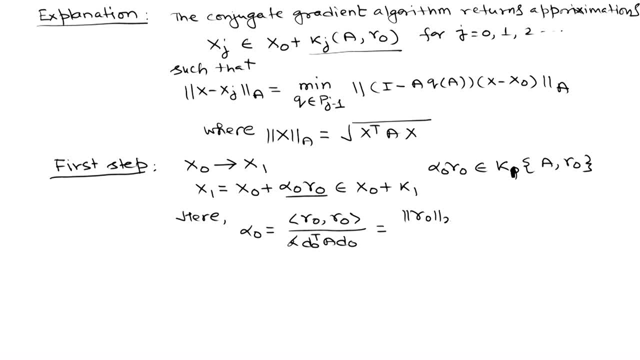 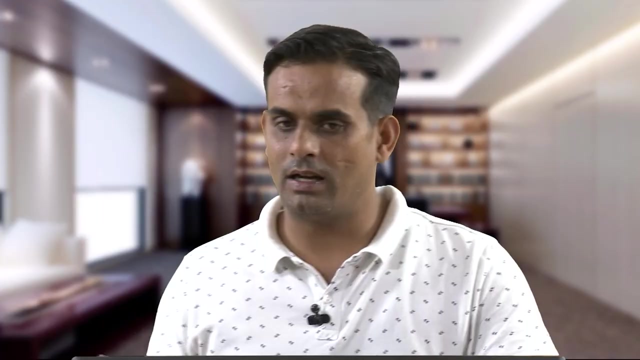 nothing, just the square of the norm of r 0 upon square of the norm induced by the matrix A on the vector d 0, and it cannot be 0, because r 0 is not 0. once r 0 is 0, method will not. 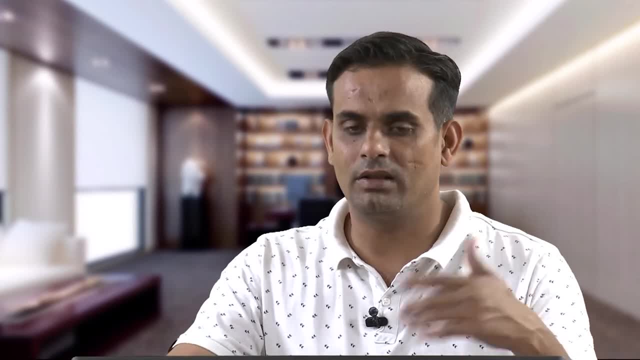 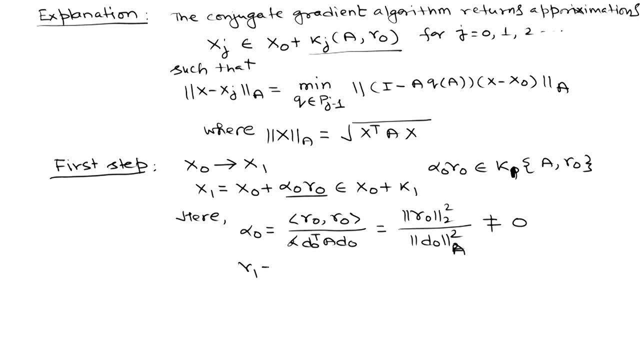 proceed. That is the termination or stop motion, Stopping condition for the conjugate gradient method. Now residual r 1 will be r 0 minus alpha a, 0, d, 0 again. this will become a vector in the second Krylov subspace of A and B. Here if r 1 is 0, then method will stop. otherwise 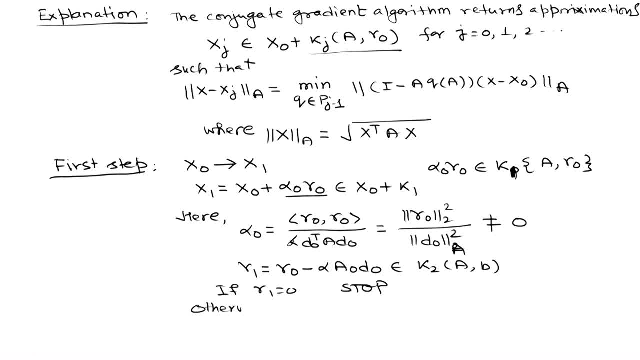 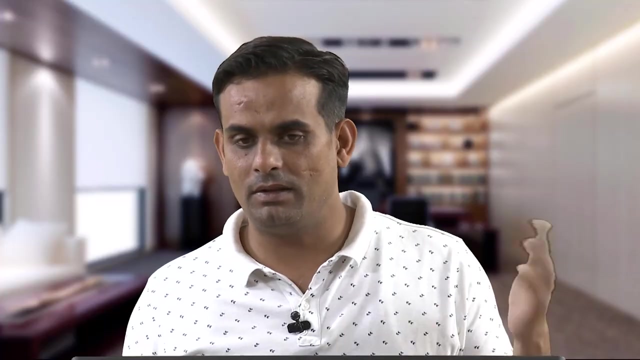 r 0, r 1 is an orthonormal basis of k 2, A, B, which is the condition when I told you about four methods. So each time the residual r j will be the will be a vector which is orthogonal to the. 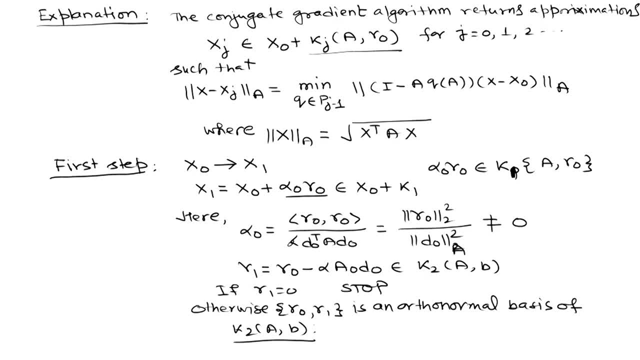 z Krylov, subspace of A and r 0.. So in this way again, when I will calculate r 2, then r 0, r 1 and r 2 will form an orthonormal basis for k 3, A, B and so on. 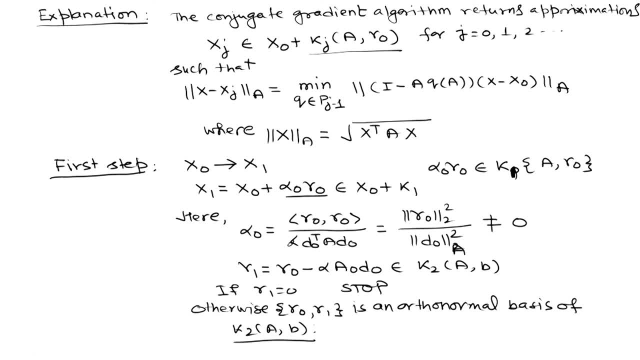 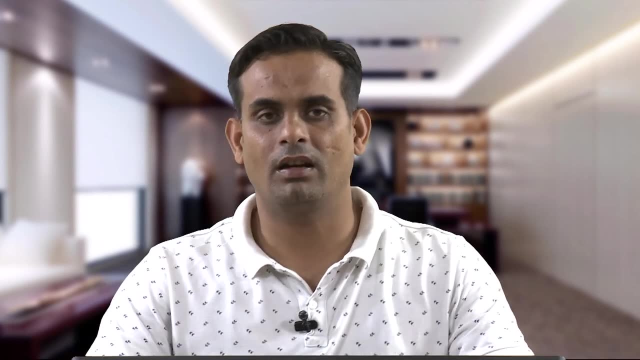 So in this way we will proceed for subsequent iterations in conjugate gradient method. So in this lecture we have learned the definition of Krylov subspace. then we have seen the motivation of using Krylov subspaces for solving large and sparse linear systems. 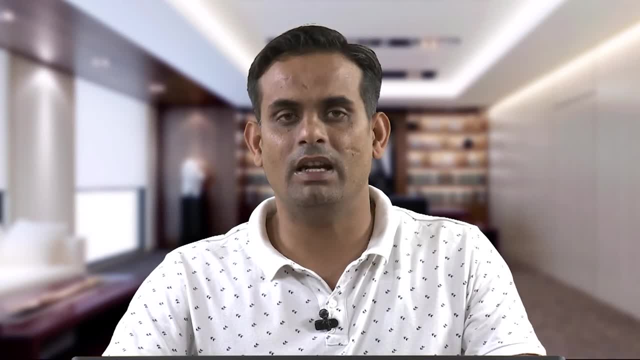 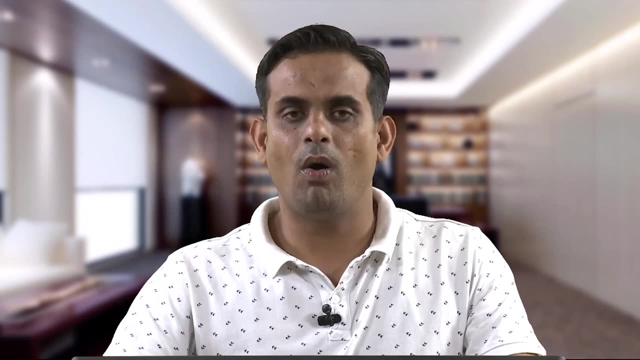 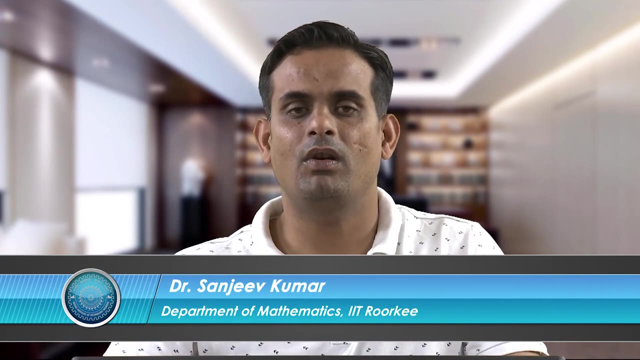 In the last phase of this lecture we have learned the conjugate gradient algorithm. In the next lecture we will take an example of conjugate gradient method. then we will see some conditions for the convergence of this method Later on in the next lecture. 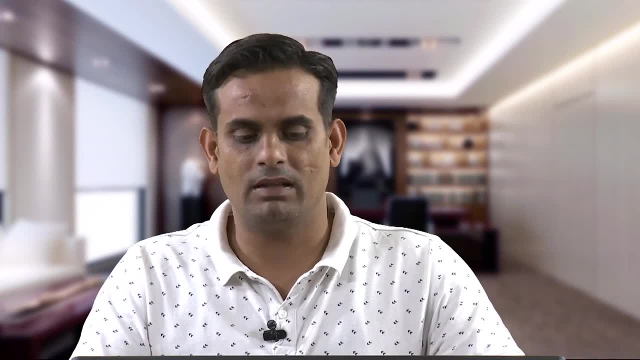 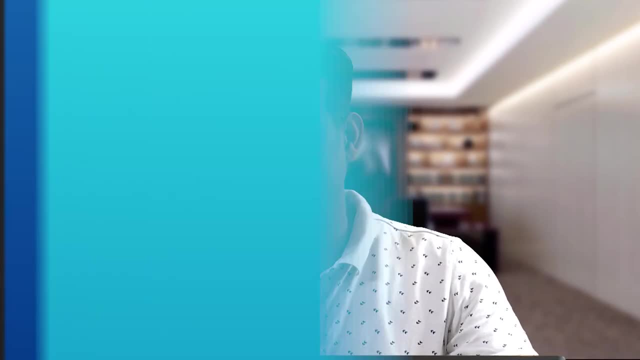 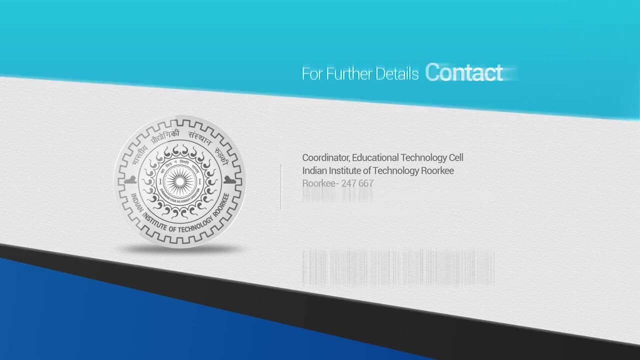 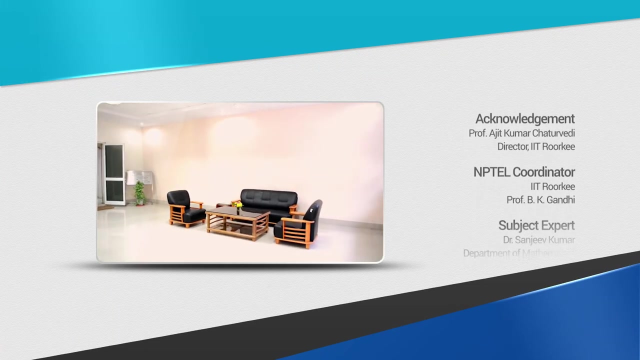 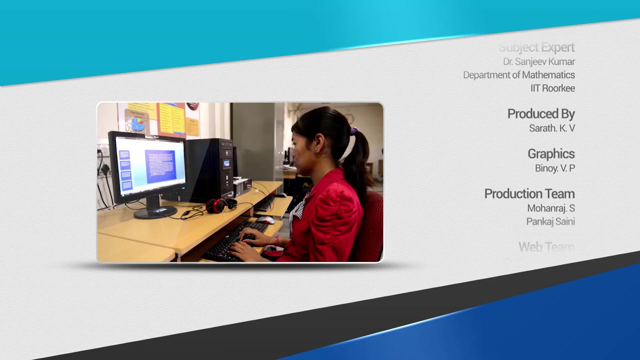 we will learn preconditioning of conjugate gradient method. These are the references for this lecture. Thank you very much. Thank you.